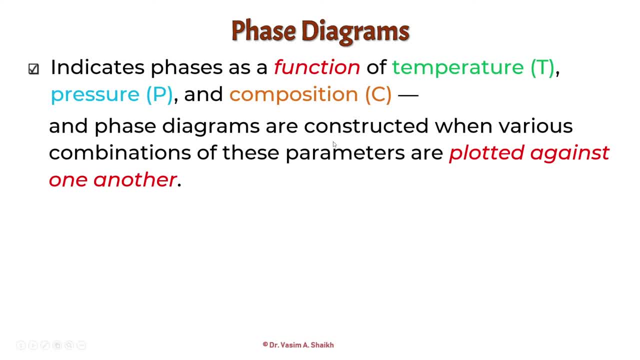 So generally the temperature and composition are varied and pressure is kept constant and based on the composition and temperature we see the different phases on phase diagram and mainly there is one important phase diagram which is the phase diagram Which is most of the time asked in the exam and we will discuss mainly on that is a binary phase diagram and the independent variable here are temperature and composition and always the pressure is kept constant, which is one atmospheric pressure, and we are making the binary phase diagram and there are different types of phase diagram, like unary phase diagram, binary phase diagram and ternary phase diagram. 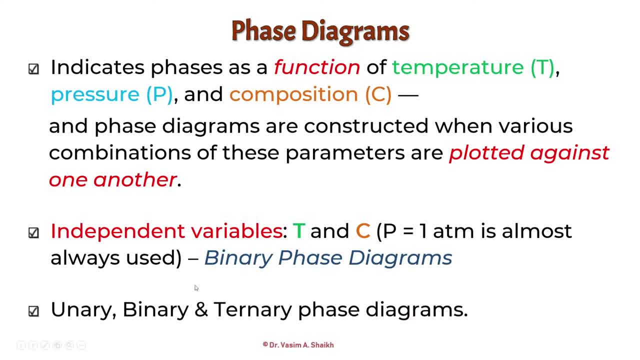 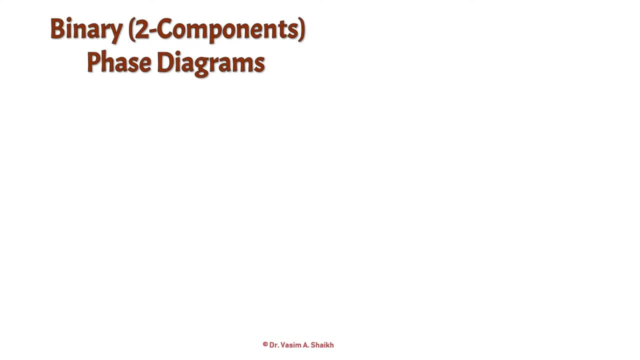 So I have discussed about what are these types of phase diagram in an earlier video, which is different types of phase diagram. So now let us move on and see what is a binary two-component phase diagram and, as we are progressing in this video, we will talk about what is an isomorphous phase diagram as well. 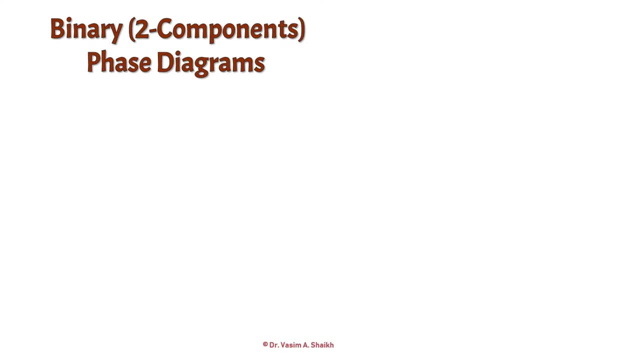 So before we start with binary phase diagram, we should know that binary means it is a two component phase diagram. so there are two components which are involved in making this phase diagram in unary phase diagram. it is one component phase diagram, the ternary phase diagram. 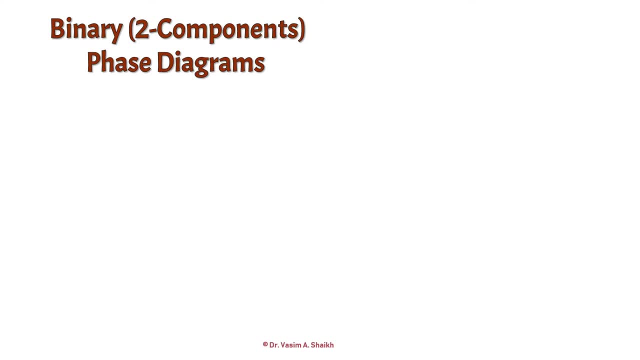 has three components, but binary is a two component phase diagram and mainly when we are studying about phase diagram, we are discussing about binary two components phase diagram. and here, for example, when we are discussing about binary phase diagram, i'll take an example of a copper nickel system. so 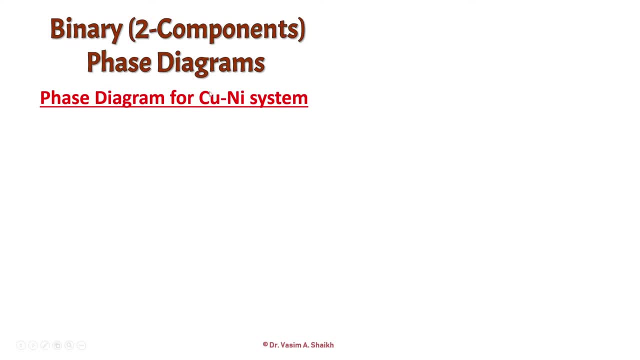 here you can see. binary means it has copper and nickel. so these are the two components of this binary phase diagram. and now let us look at a phase diagram of copper and nickel. so here on the x-axis you can see, we have the composition. the composition is there on the x-axis and here. 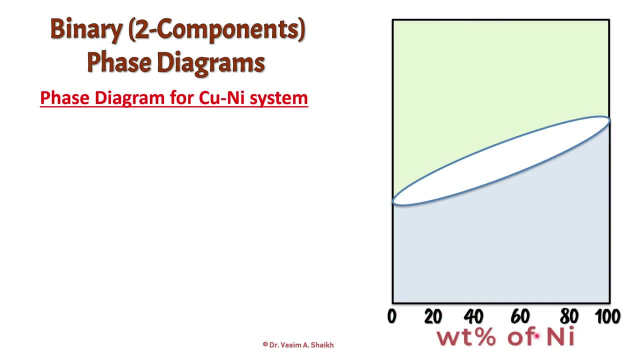 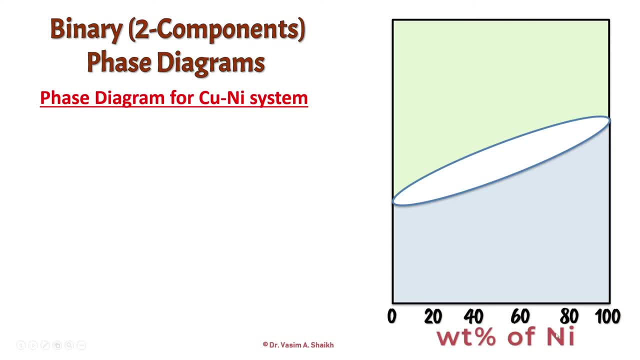 are increasing the weight percent of nickel. the weight percent of copper is decreasing. so here we have 100 percent copper and here we have 100 percent nickel. so this is 100 percent copper and this is 100 percent nickel, and on the y-axis we have temperature. so here we are, starting with 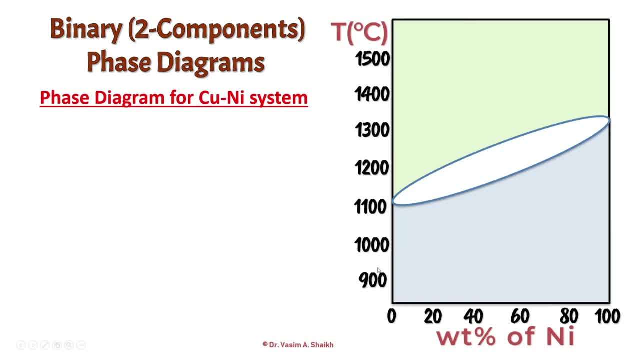 we are starting with 900 because below this the phase is same, so we are not bothered about what is below 900, and because the phase change will take place beyond 1100 degree Celsius. so we are starting with nine hundred and not with zero. so you can imagine from nine hundred to zero. 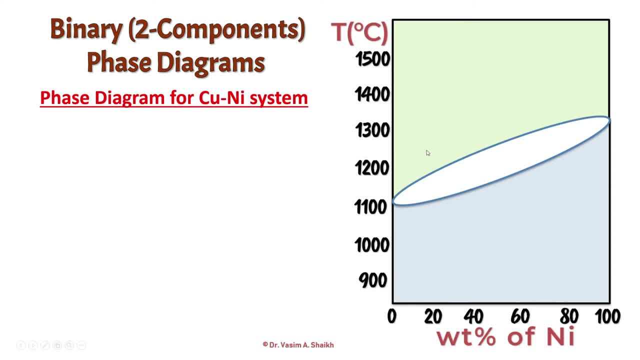 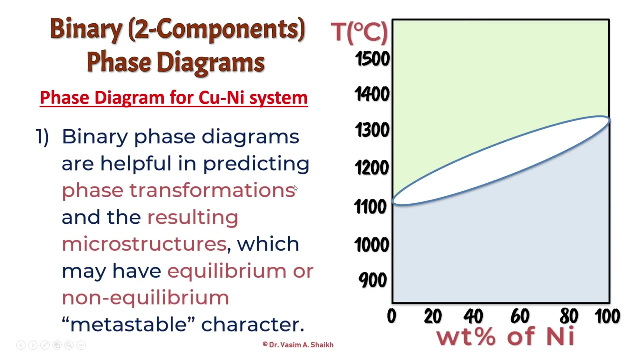 the phase is same, so we'll discuss about what are the different phases on this phase diagram. so it is going from 900, 1100, 1200, 1300, 1400 and 1500 and this is temperature in degree celsius. so degree c is celsius or centigrade. then the binary phase diagrams are helpful in predicting the phase. 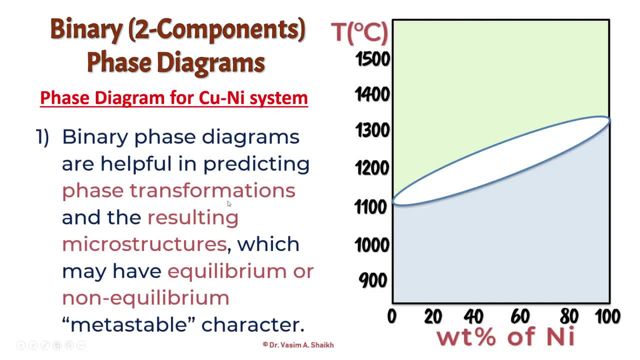 transformation and the resulting microstructures which are there, which may have equilibrium or non-equilibrium, metastable characteristics. so here in this binary phase diagram, we can see that the different phases are there. for example, this phase which is in green color- light green color- is a liquid phase, okay, and this blue color phase is a solid phase. so we know that phase diagram. 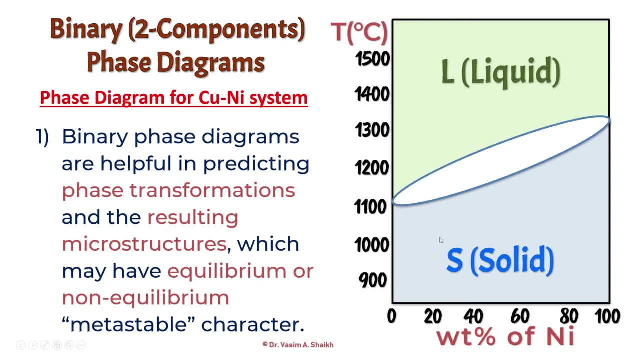 in a phase diagram we can predict or see what are the phases existing at different temperature and composition. so this is a liquid phase, this is a solid phase. and this solid phase, they have given it a name as a alpha, so this is called as an alpha phase, and in between we have both the phases, which are 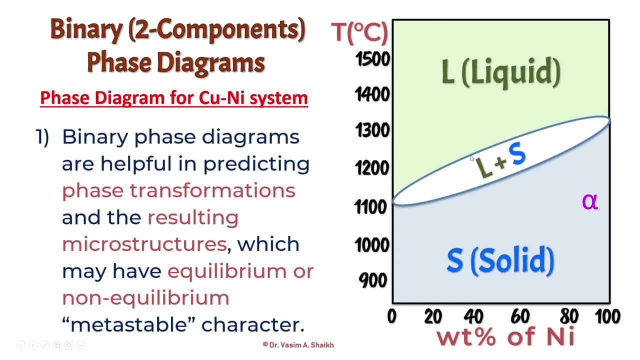 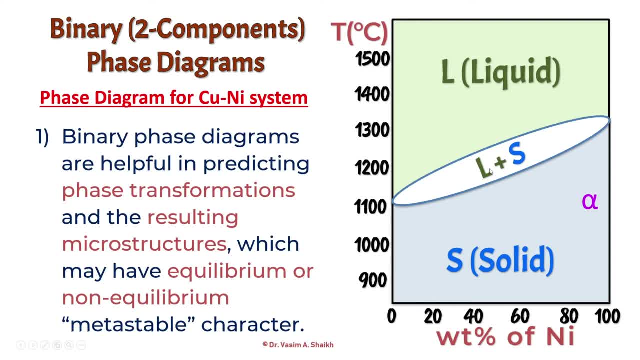 where you will have both the phases. so here we will have both the phases of liquid plus solid. so where you will have both the phases. so here we will have both the phases of liquid plus solid. so where you will have both the phases. so here we will have both the phases of liquid plus solid. so l is liquid and this is. 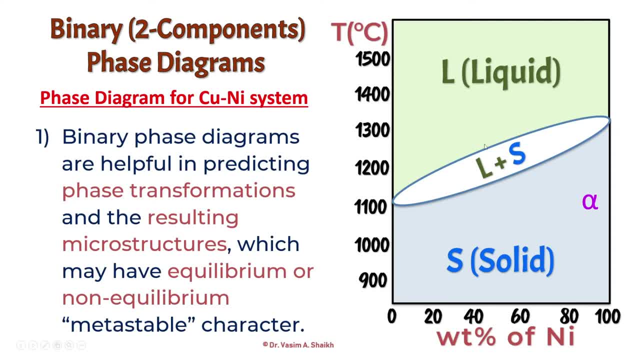 here we will have both the phases of liquid plus solid, so l is liquid. and this is here. we will have both the phases of liquid plus solid, so l is liquid and this is solid. so in between, if you are in between, solid, so l is liquid and this is solid. so in between, if you are in between, 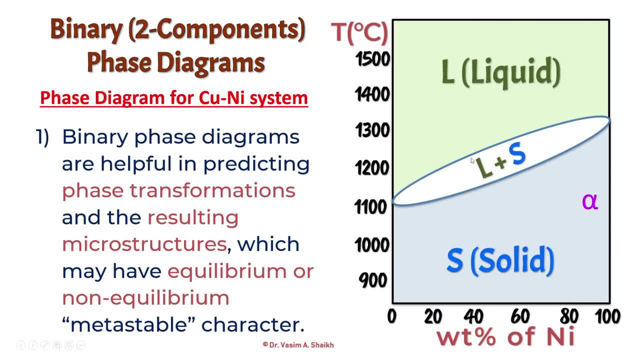 solid. so l is liquid and this is solid. so in between, if you are in between, this phase field, it is called as a phase, this phase field, it is called as a phase. this phase field, it is called as a phase field. you will have liquid and solid, so both. 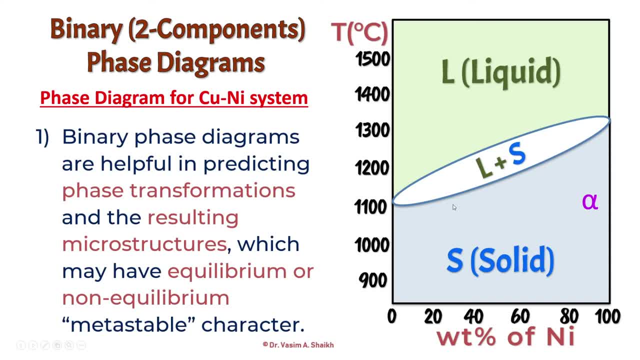 the phases will be present, and this is called as the liquidus line. this is the liquidus line, and the meaning of the liquidus line is that anything above the liquidus line is liquid. so anything above the liquidus line, this green area, is liquid. similarly, we have a solidus line. 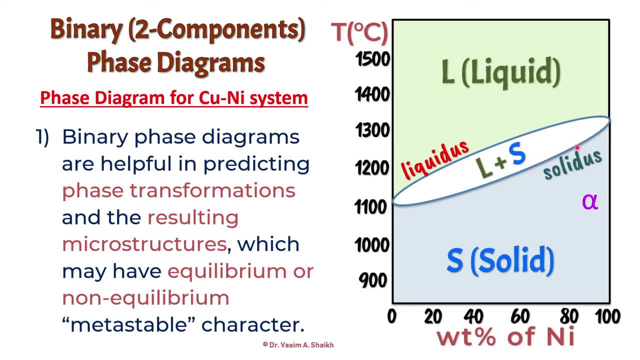 so below the solidus line, this is the solidus line and below the solidus line, anything which is there, any phase existing, is a solid phase. so that we have to remember, this is the definition of a liquidus and the solidus line. anything above the liquidus line is liquid, anything. 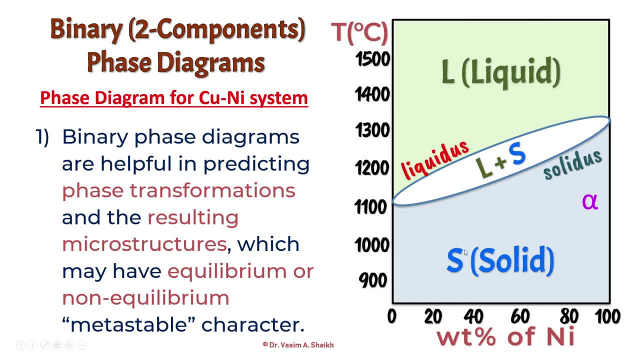 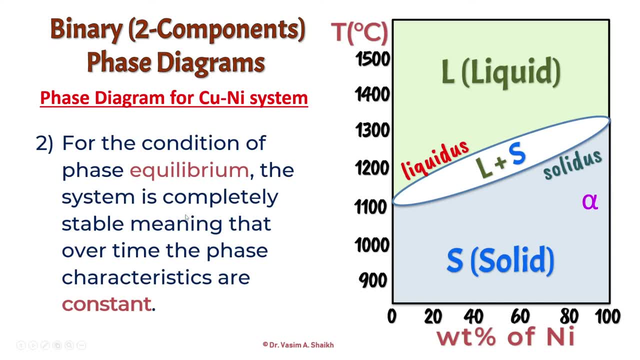 below the solidus line is solid. so for the condition of equilibrium the system is completely stable, meaning that over time the phase characteristics are constant. so we call this phase diagram as an equilibrium phase diagram as well. so why we call it as an equilibrium phase diagram? because these phases, over time they will 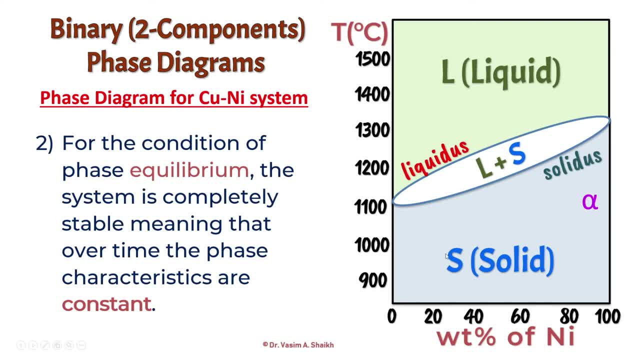 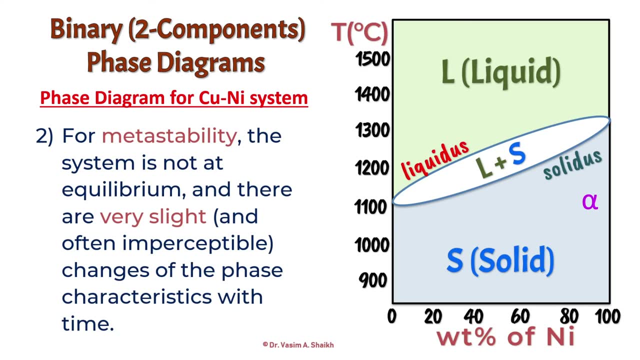 not change. so we are assuming that even as the time is passing by, the phases will not change and it will be constant. so that is the meaning of it is in a equilibrium condition. but for meta stability, system is not at equilibrium and there are very slight or sometimes imperceptible changes of the 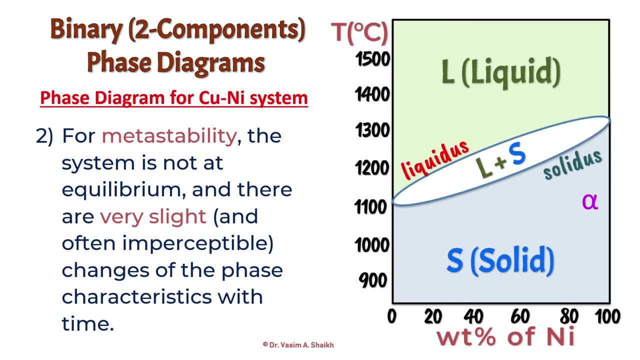 phase characteristics with time. so suppose if we say that this phase is a metastable phase, that means we are assuming that after some time the phase might change. but these changes are very slight and even by naked eye we can't see these changes. so but sometimes we say that you know it.